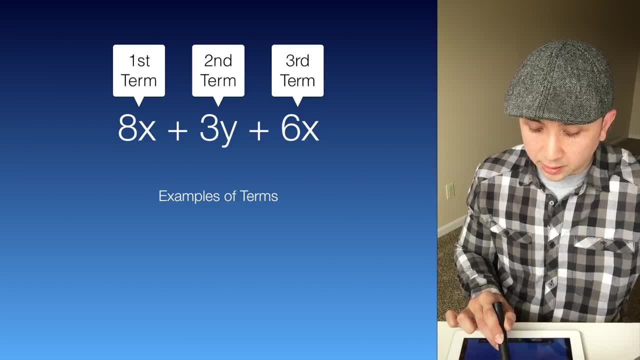 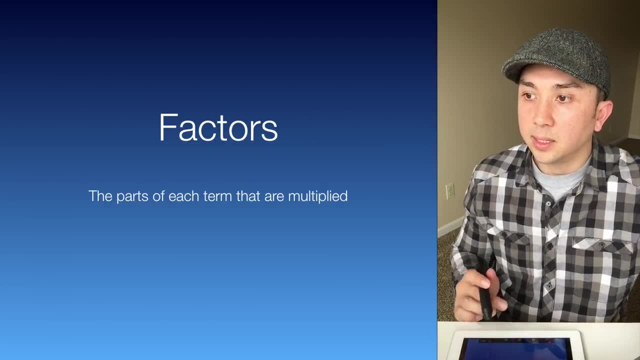 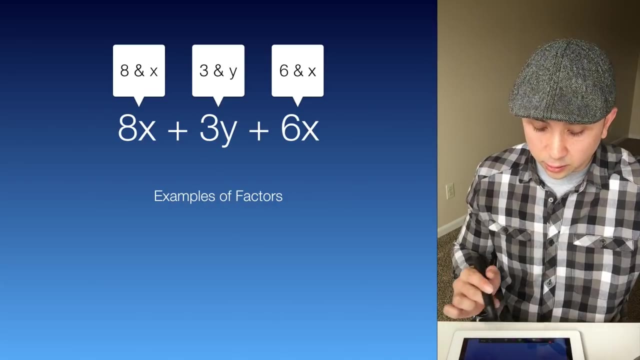 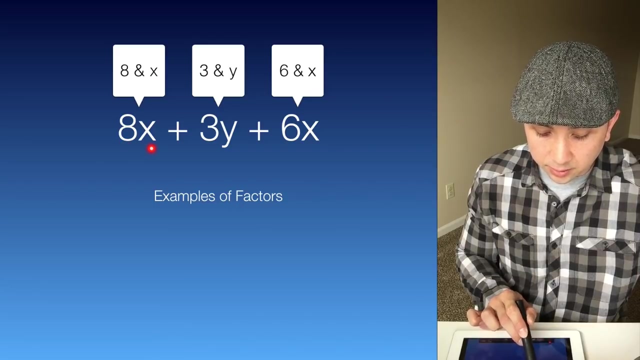 Our second term is 3y, separated by addition, and our third term is 6x. Now factors are the parts of each term that are multiplied. So here we can see that in the first term our factors are 8 and x. because 8 and x 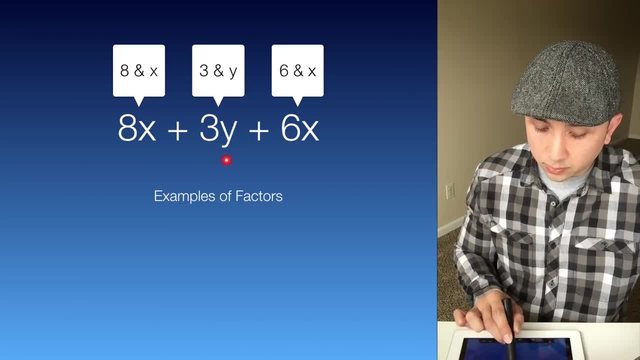 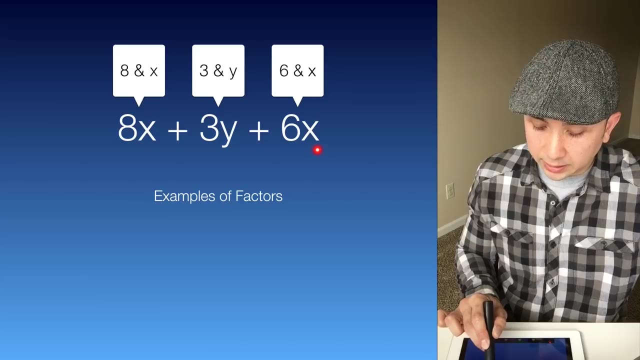 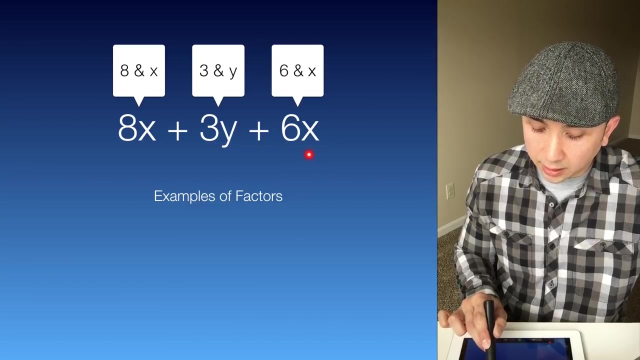 are being multiplied. So in our second term, 3y, our factors are 3 and y because 3 and y- y are being multiplied, And in our third term, 6x, our factors are 6 and x because 6 and x are being. 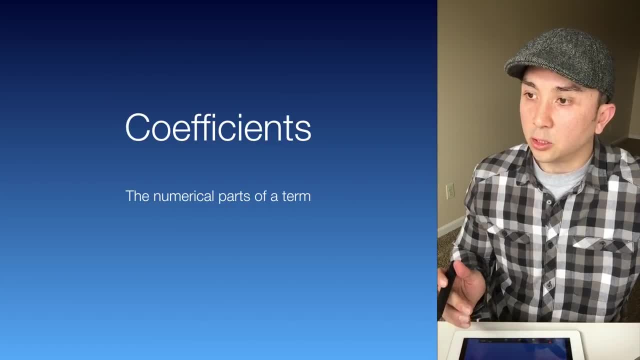 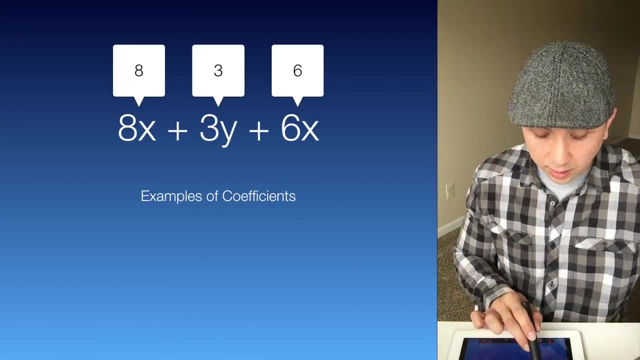 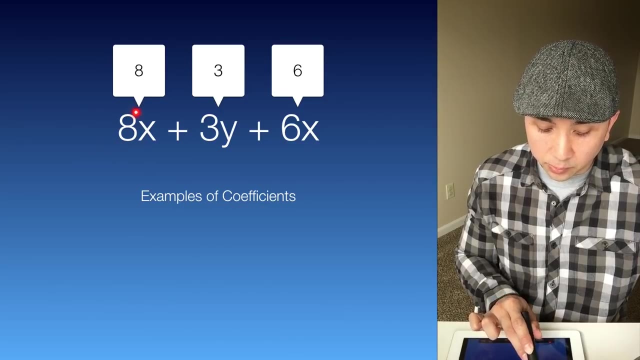 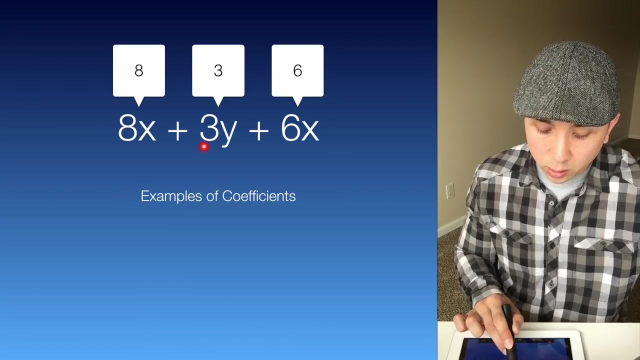 multiplied. So coefficients are the numerical parts of a term. So here in our first term, our coefficient of 8x is 8. It's just the numerical part of a term. So here in our second term, 3y, our coefficient is 3.. And in our third term, 6x, our coefficient is 6.. Now, like terms, 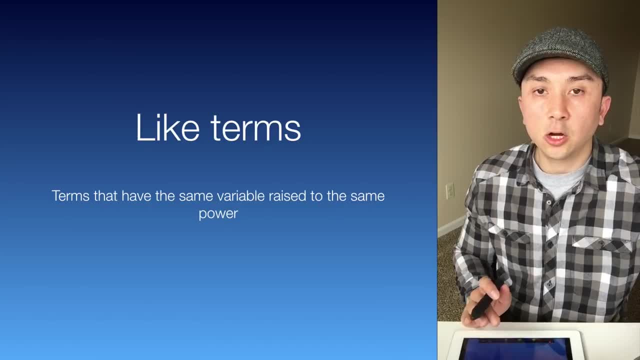 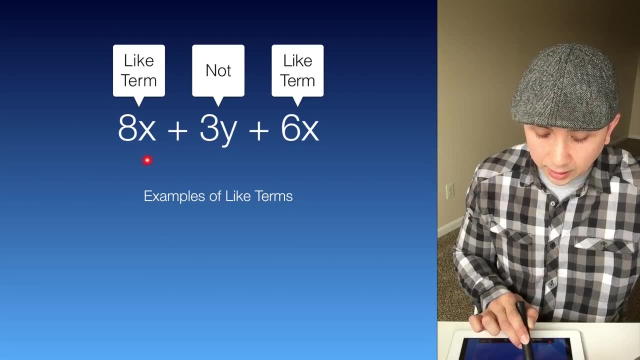 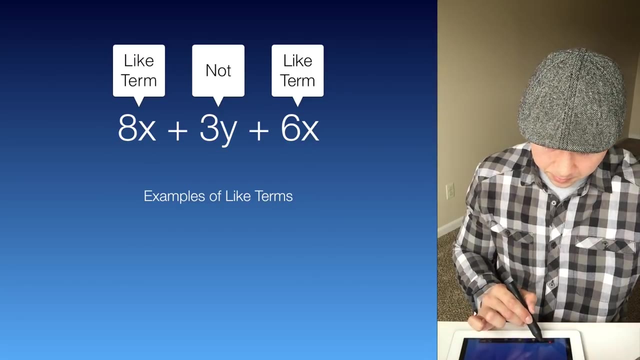 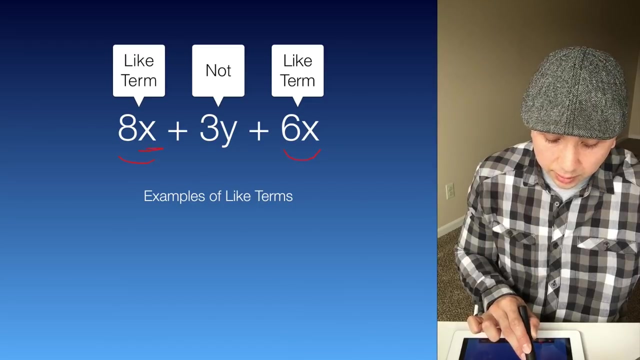 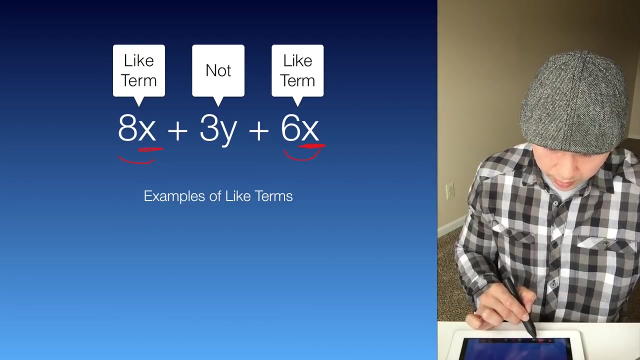 are terms that have the same variable raised to the same power. So here we have 8x, 3y and 6x. Now 8x, 8x and 6x are like terms because they share the variable x raised to the first power. Now 3y is not a like term because 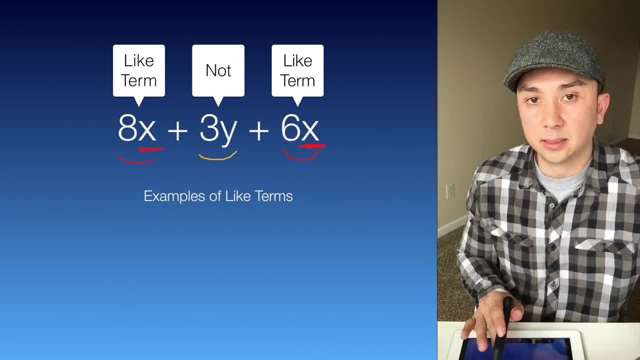 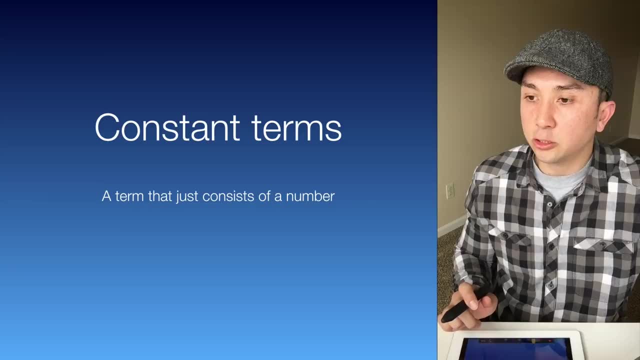 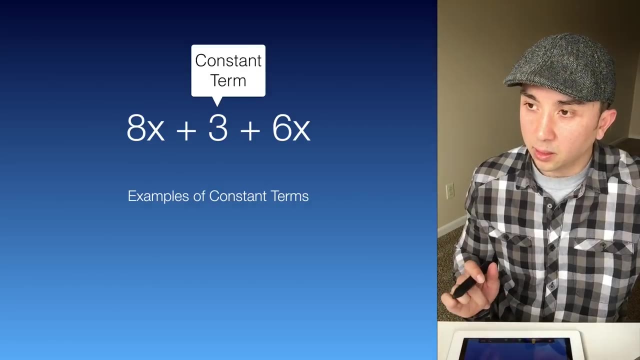 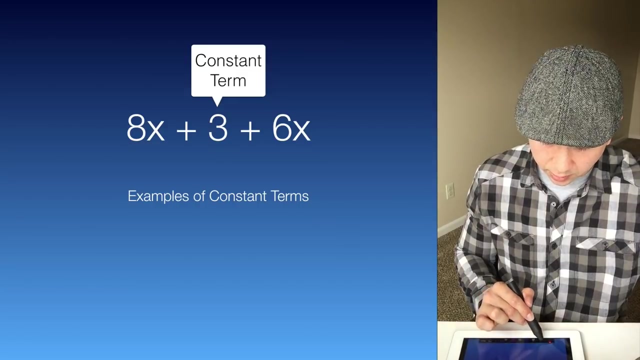 it has the variable y and not x, So it is not a like term. Now, constant terms are terms that just consist of a number. They just have a number and that's it. So here we can see that in our second term we just have 3.. So that means 3 is a constant term because it just 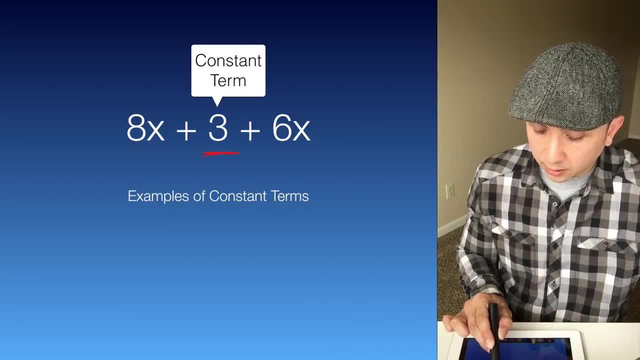 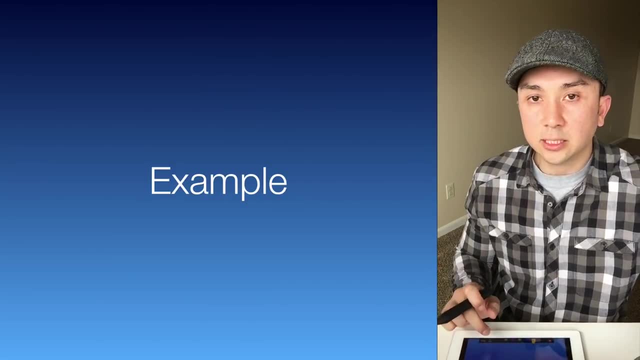 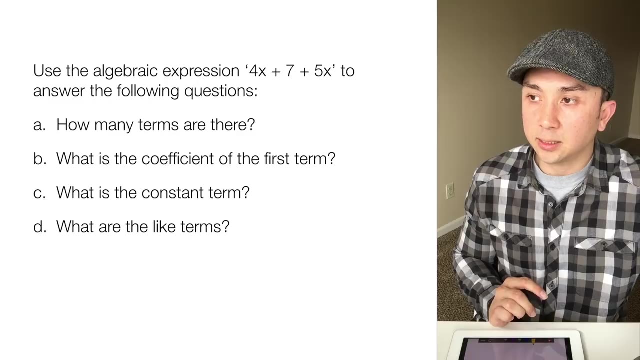 has 3.. It does not have a variable or anything attached to it, It just has 3.. So let's do an example. So use the algebraic expression 4x plus 7 plus 5x to answer the following questions. 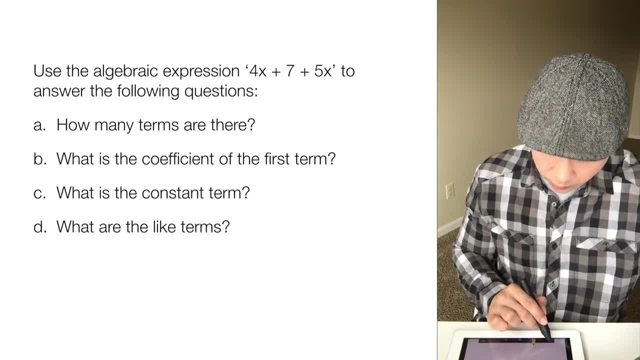 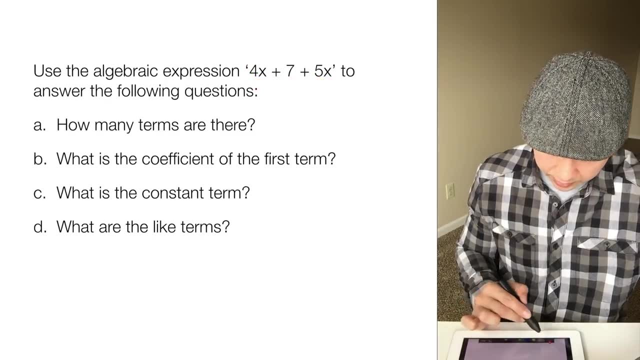 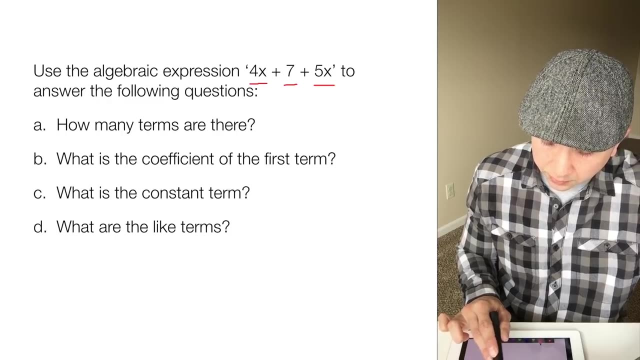 How many terms are there? Well, we can see that we have 4x, 7, and 5x. So here's our first term, there's our second term and here's our third term, And they're being separated. 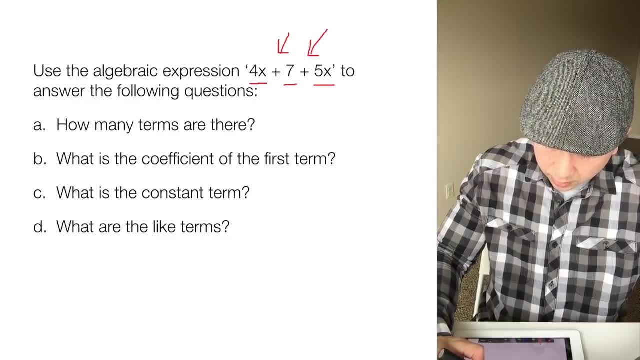 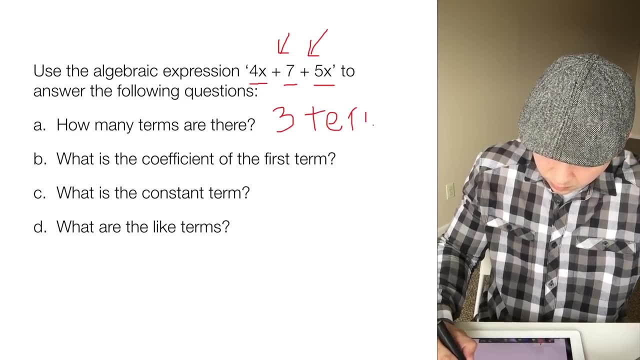 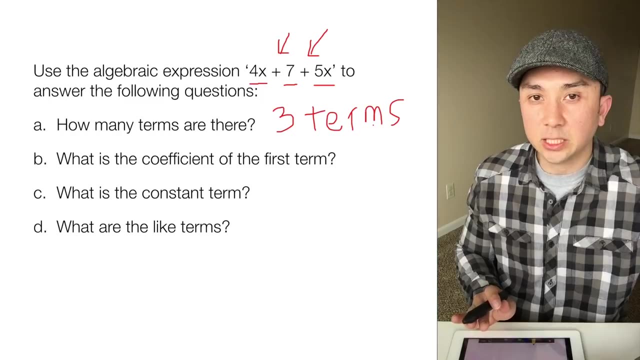 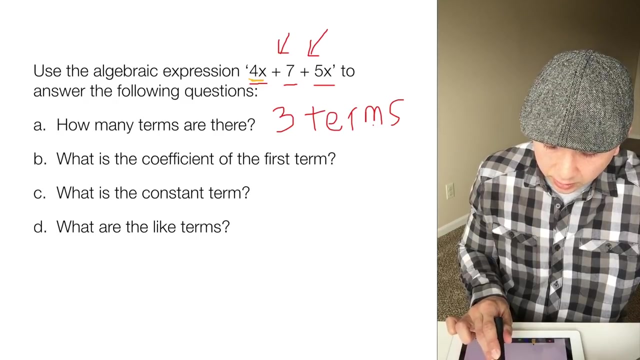 by the addition sign. So we have 3 terms. So what is the coefficient of the first term? Remember, coefficient is just the number in front of a variable, It's only the number. So here we can see: 4 is our coefficient of the. 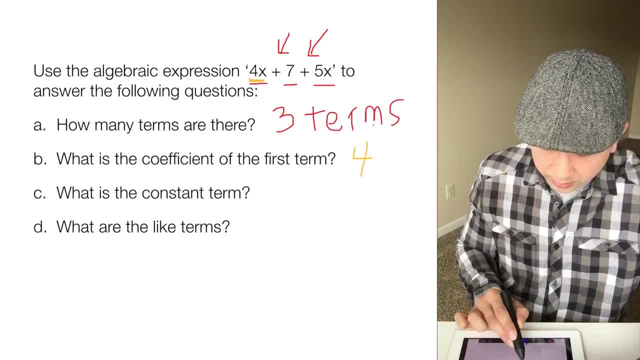 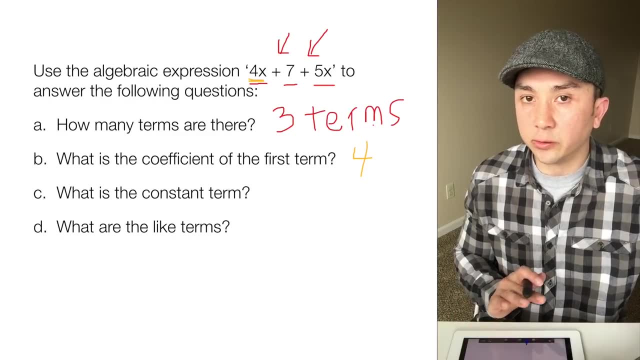 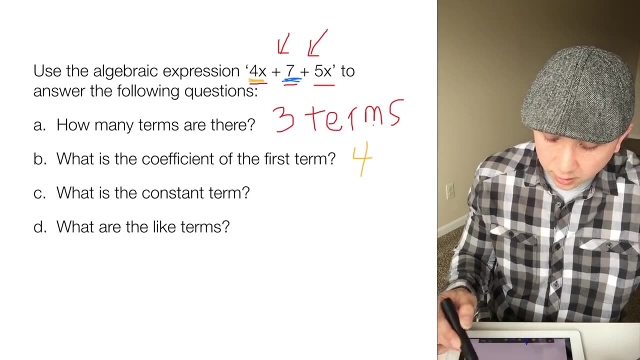 first term. So what is the constant term? Now, remember, a constant term is just a number. It does not have a variable or anything attached to it. So let's do an example. So here we can see that 7 does not have anything attached to it. So that means: 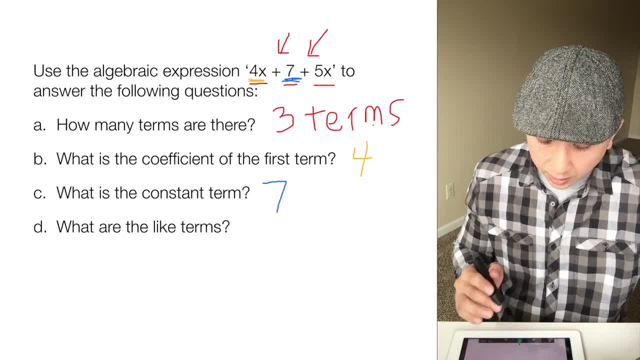 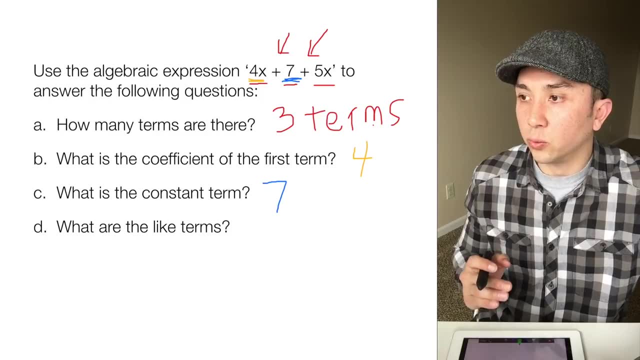 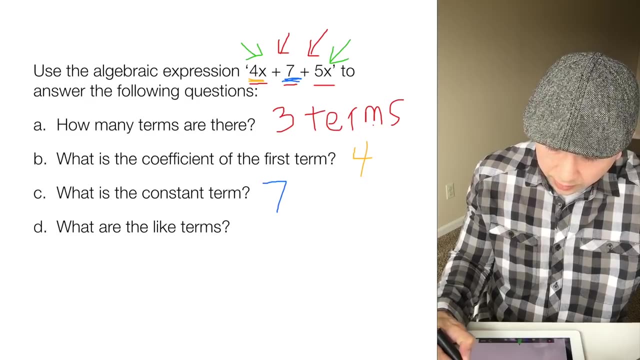 7 is our constant term. And what are the like terms? Well, like terms have a variable raised to the same power. So here we can see that 4x and 5x both have x raised to the same power. So here we can see that 4x and 5x both have x raised to the. 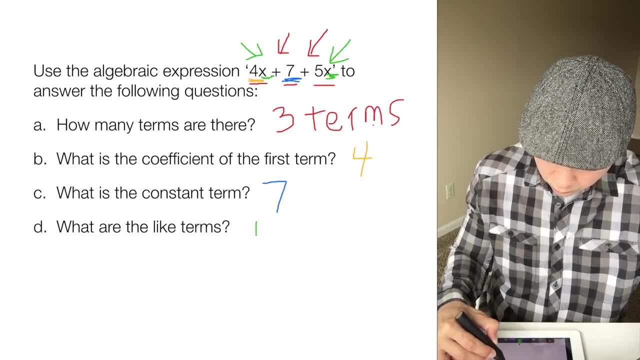 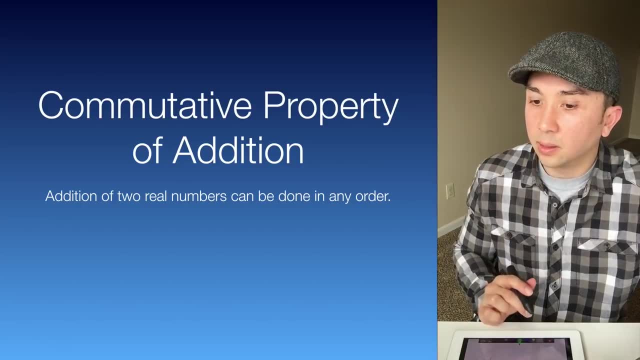 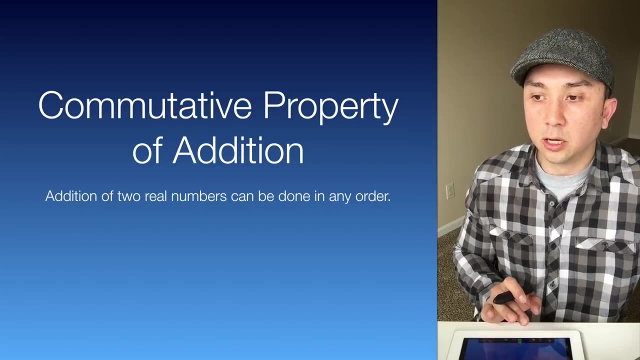 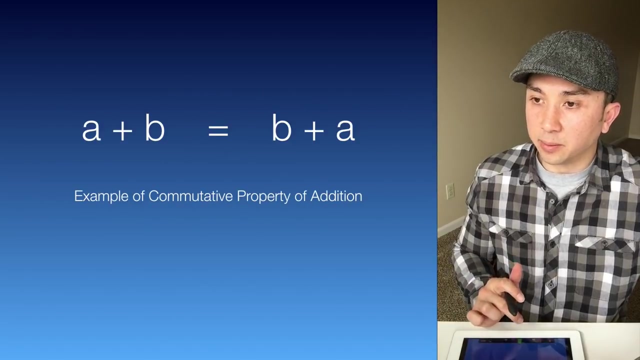 first power. So our like terms are 4x and 5x. Now the commutative property of addition states that the addition of two real numbers can be done in any order. So here's an example. So the commutative property of addition states: 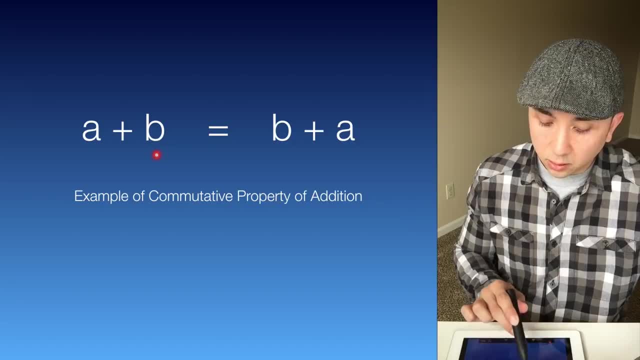 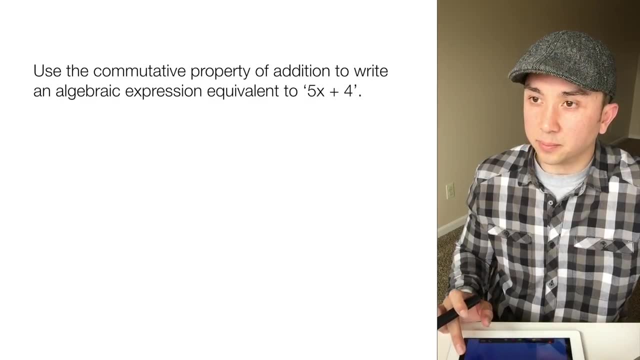 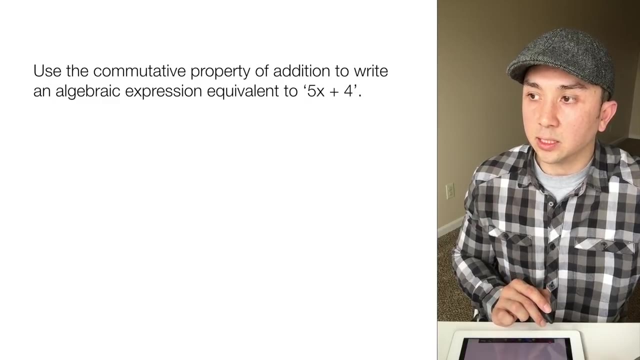 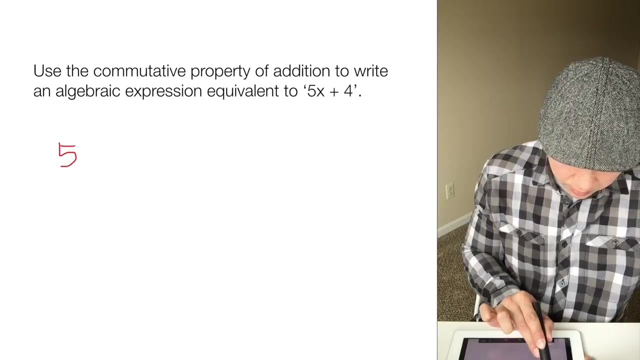 that we can either do a plus b or we can do b plus a in any order. So let's do an example. Use the commutative property of addition to write an algebraic expression equivalent to 5x plus four. So we know that we can write 5x plus four. 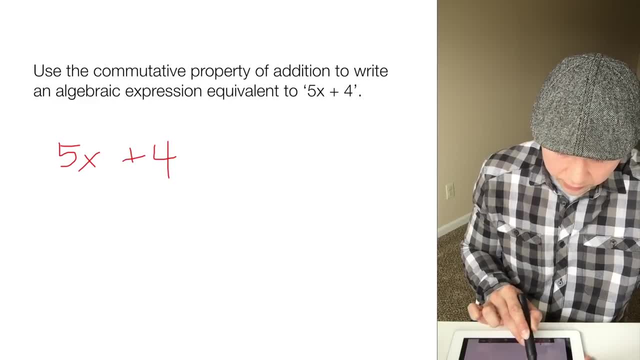 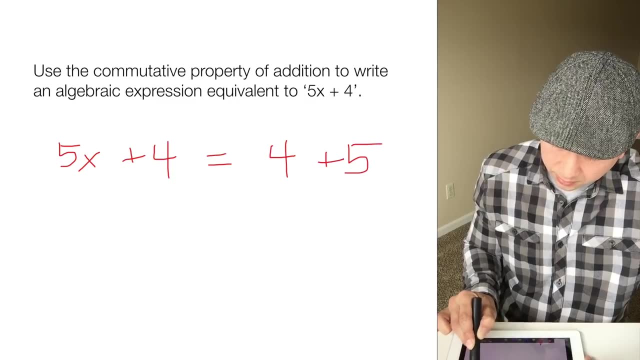 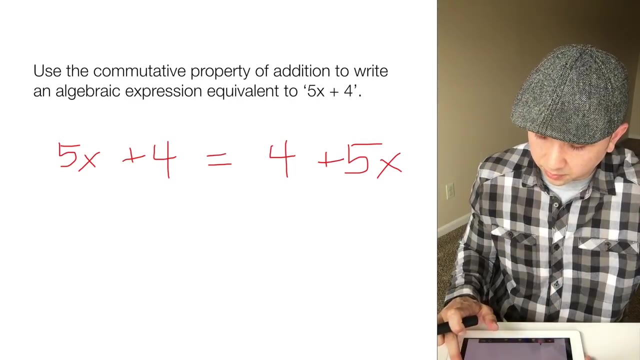 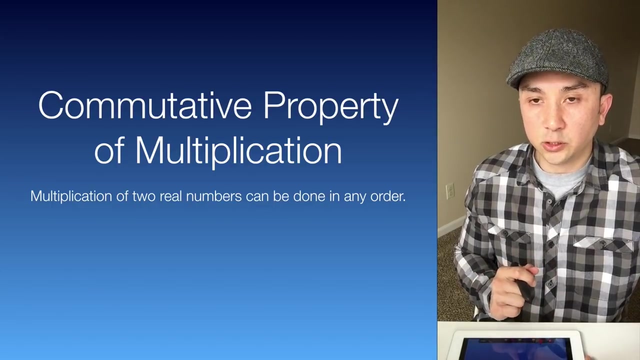 Plus four. we can add 5x plus four, or we can add four plus 5x. So that's the equivalent using the commutative property of addition. Now the commutative property of multiplication states that multiplication of two real numbers 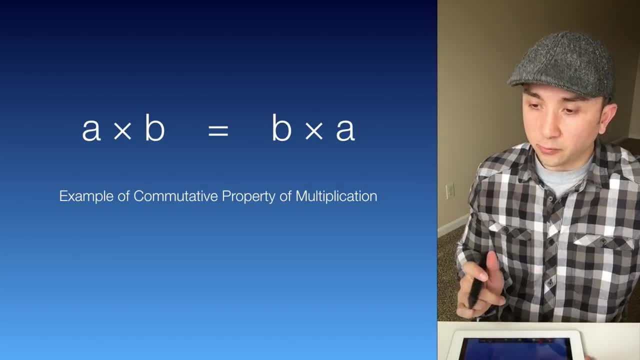 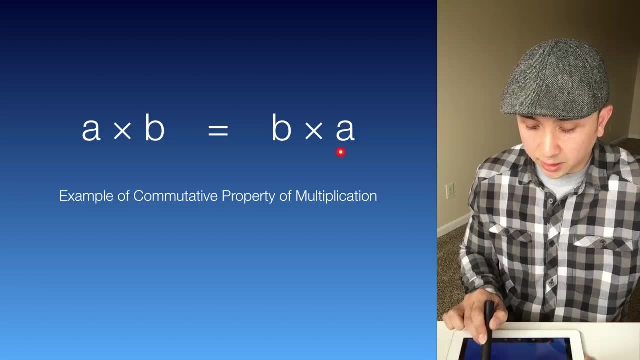 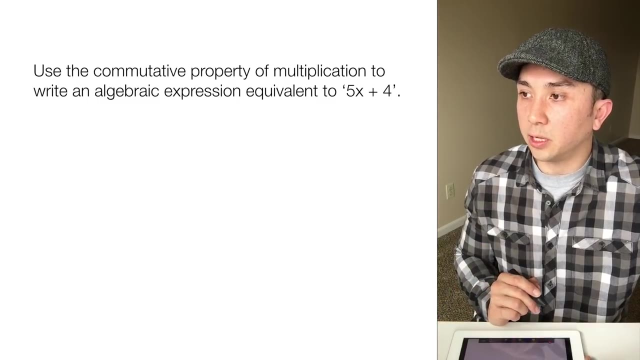 can be done in any order. So, for example, we could either do a times b or we could do b times a. So let's do an example. Use the commutative property of multiplication to write an algebraic expression equivalent to 5x plus four. 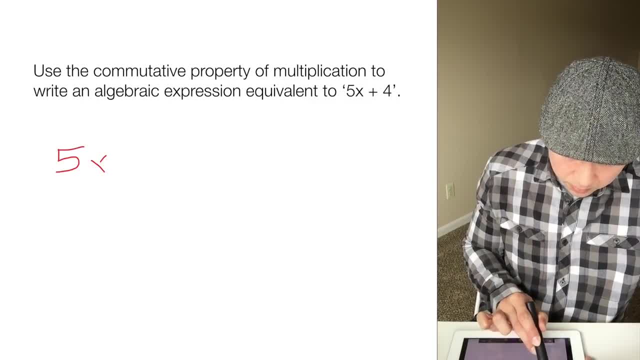 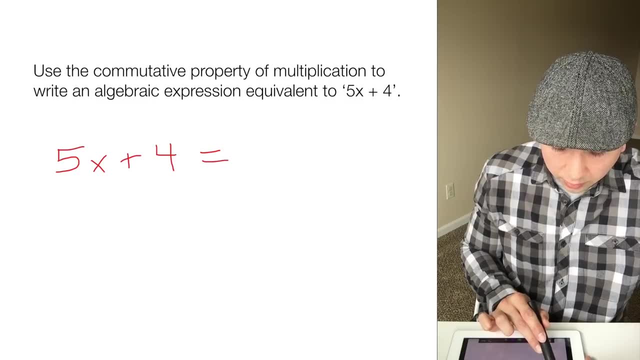 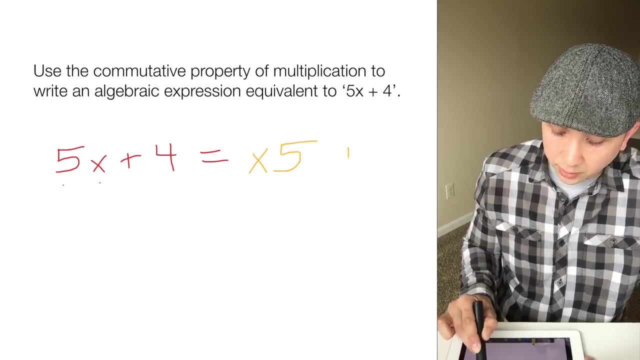 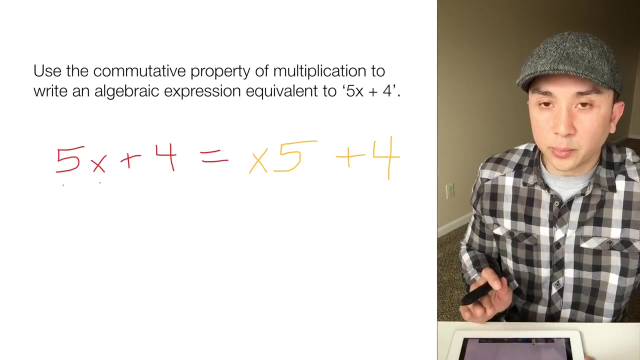 So we have 5x plus four. now we know we can multiply in any order. So we could either multiply five times x or we could do x times five plus four. So here's the algebraic expression equivalent using the commutative property of multiplication. 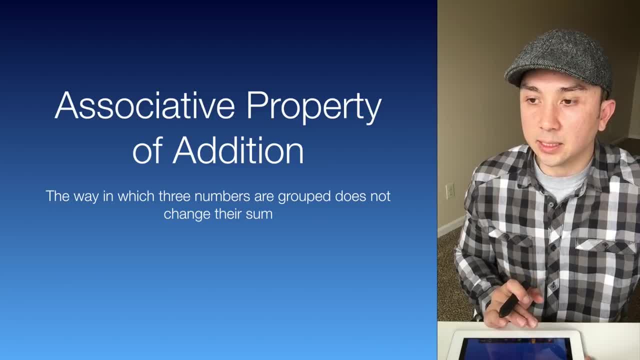 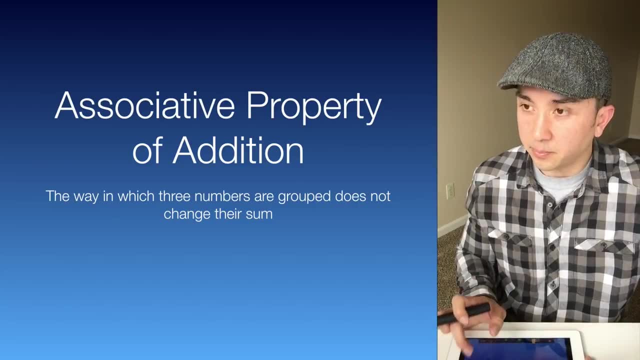 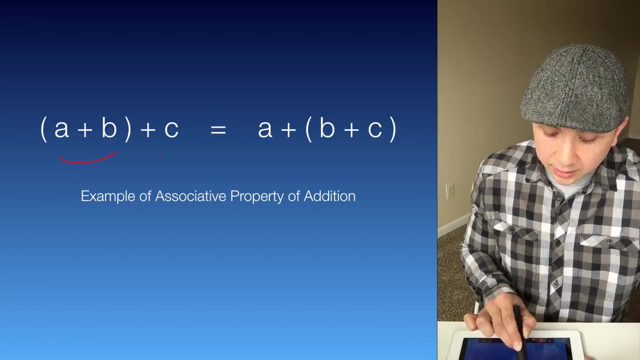 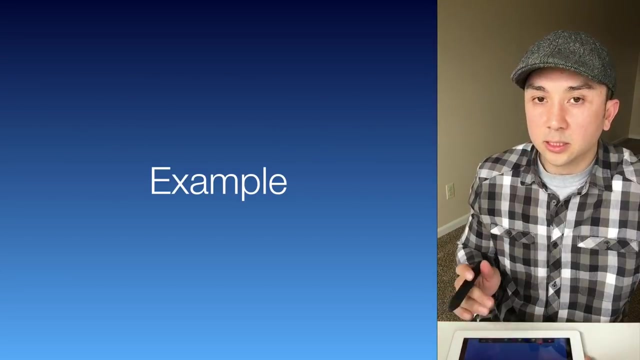 Now the associative property of addition states that the way in which three numbers are grouped does not change their sum. So we could either do a plus b and then add c, or we could add b plus c and then add a. So let's do an example. 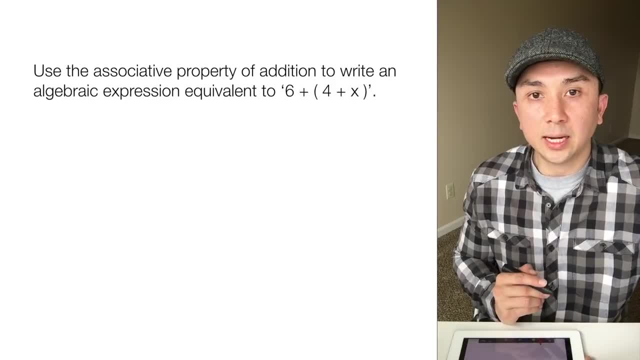 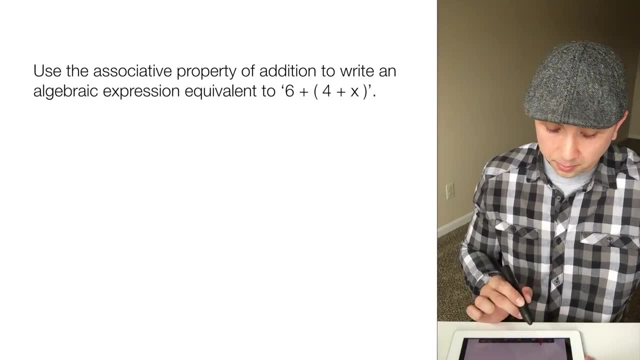 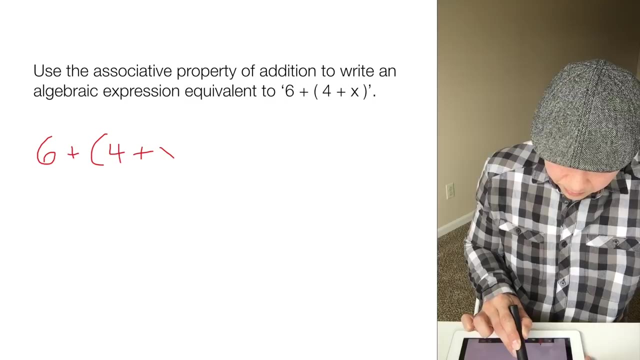 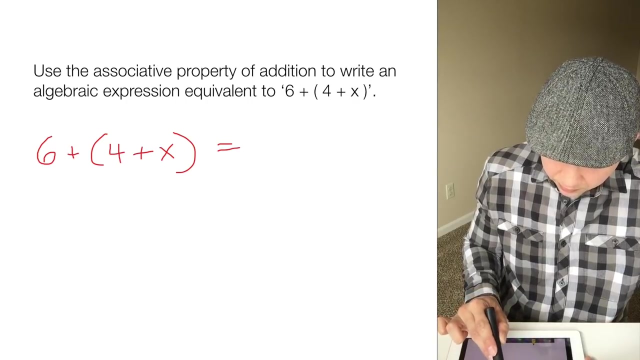 Use the associative property of addition to write an algebraic expression equivalent to six plus four plus x. So here we have six plus four plus x. Now we know we could either do four plus x, or we could do six plus four and then add x. 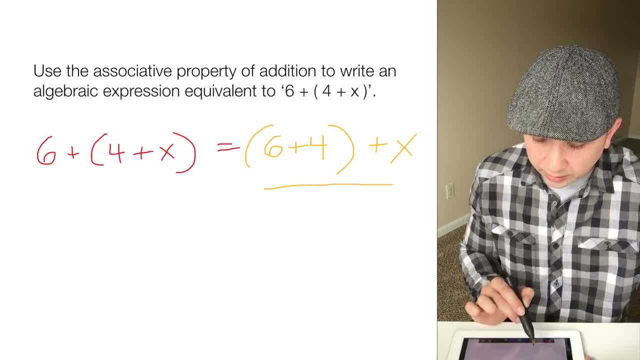 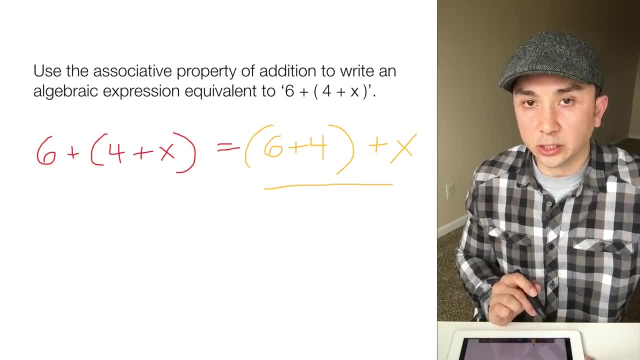 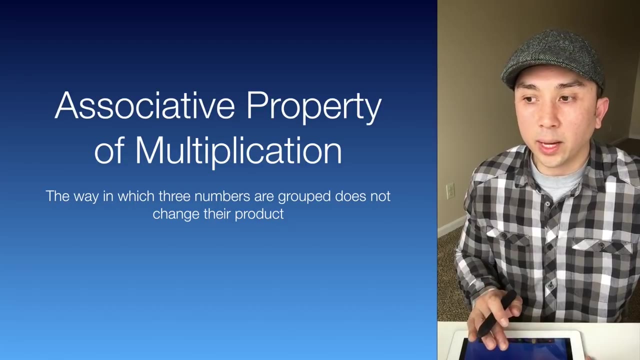 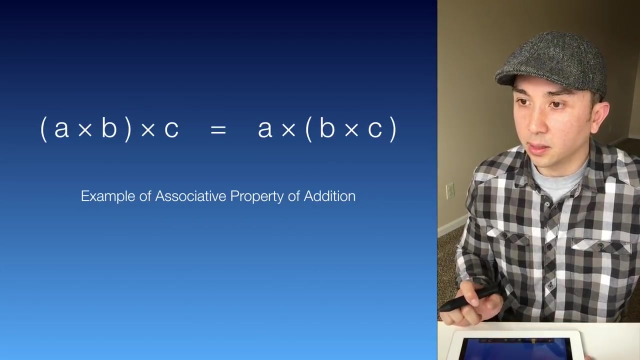 So here's the algebraic expression equivalent to six plus four plus x using the associative property of addition. Now the associative property of multiplication states that the way in which three numbers are grouped does not change their product. So for example, we could either do a times b: 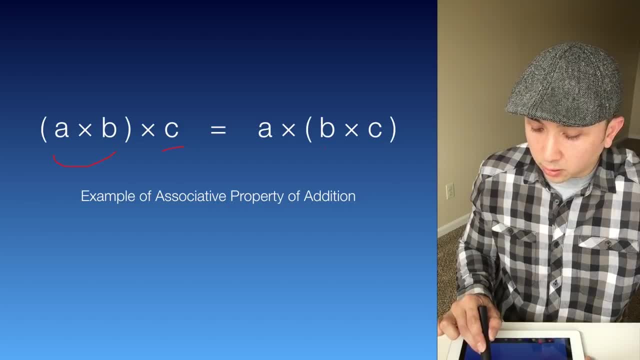 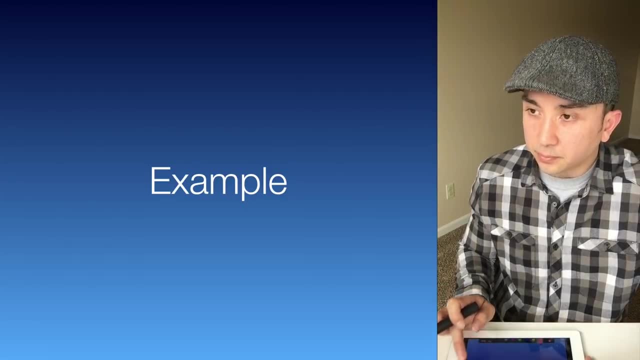 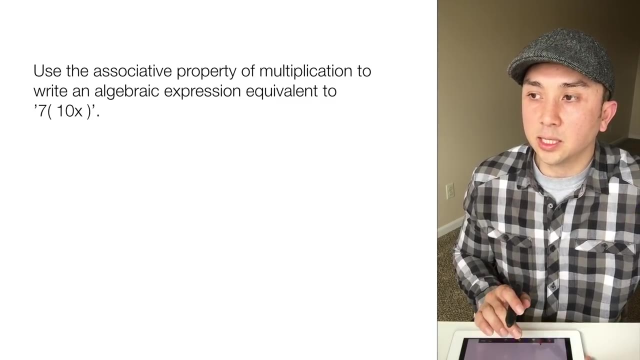 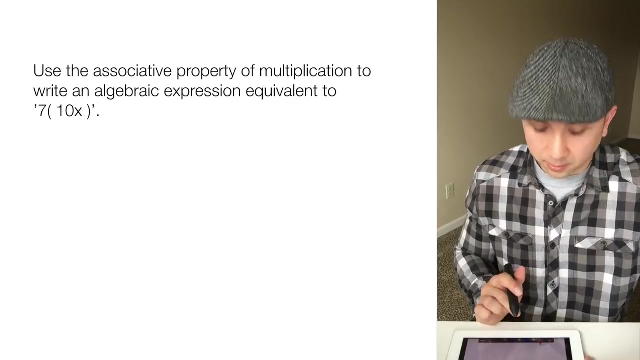 and then add c, or we could do b plus x, or we could do b times c and then add a. So let's do an example. Let's use the associative property of multiplication to write an algebraic expression equivalent to seven times 10 times x. 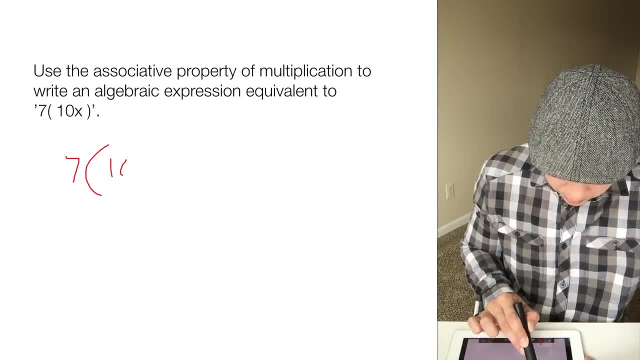 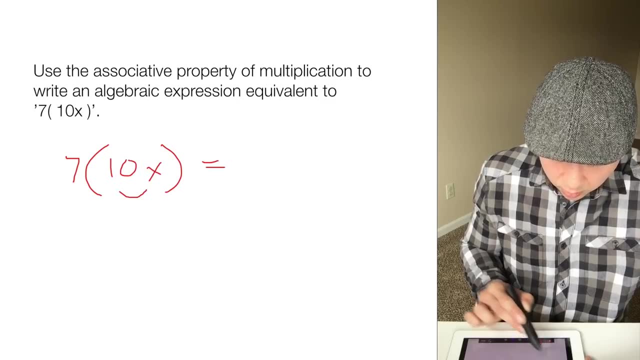 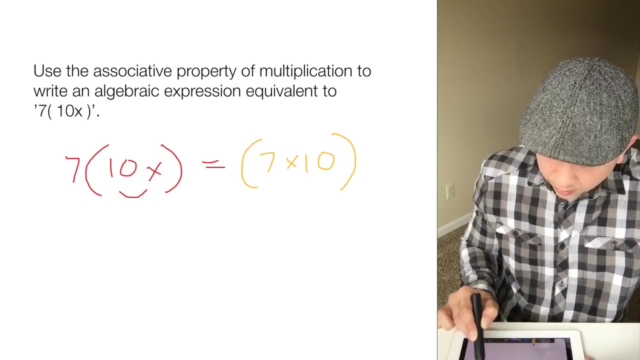 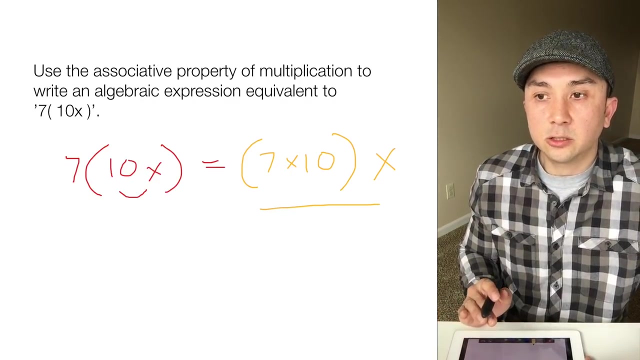 So here we have seven times 10 times x. Well, we know that we can do that right, That we could either do 10 times x or we could do seven times 10 times x. So here's the algebraic expression equivalent. 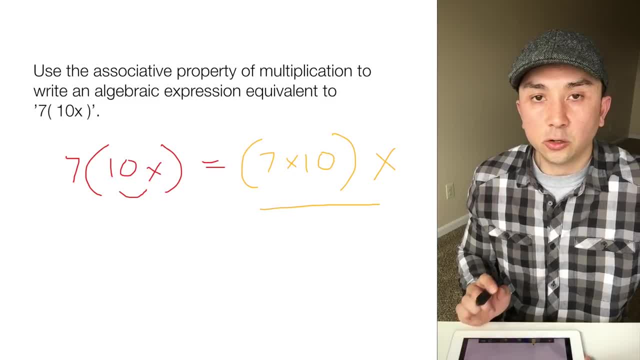 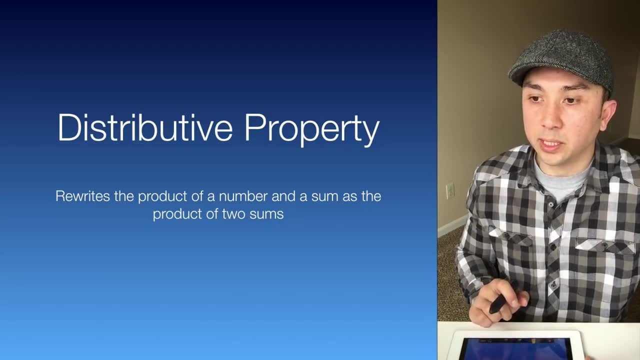 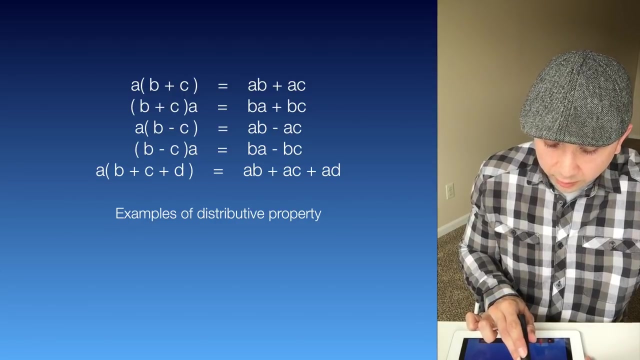 to seven times 10 x using the associative property of multiplication. Now the distributive property rewrites the product of a, the product of a number and a sum as the product of two sums. So here, for example, we have b plus c times a. 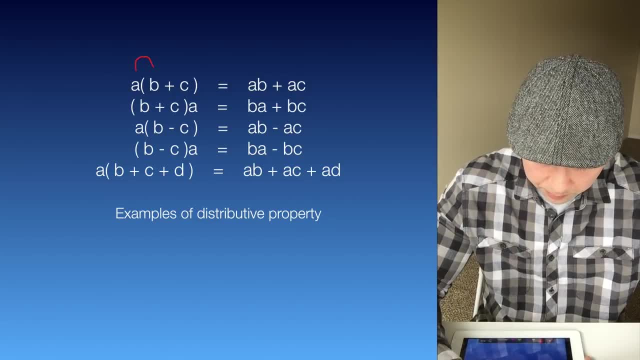 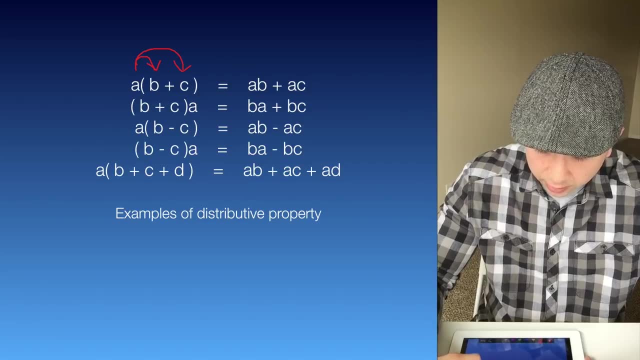 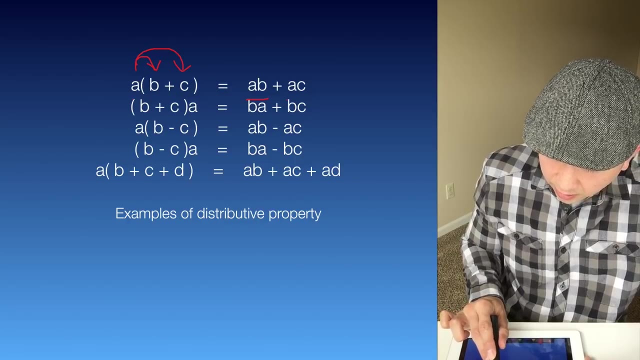 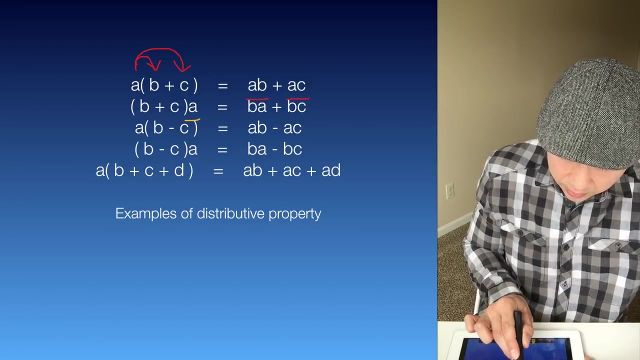 Now we, using the distributive property, we distribute a to b, and then we distribute a to c, And so when we do that we will have a times a, times b and then a times c. So here we can distribute a to b. 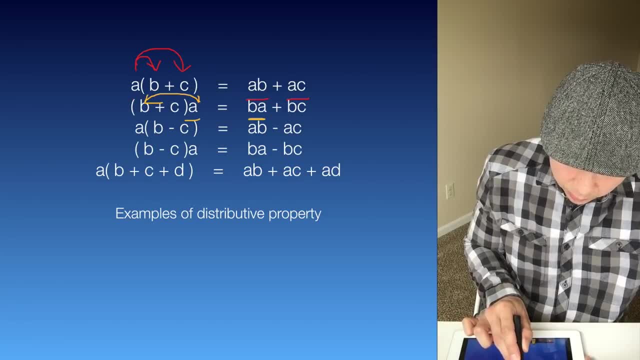 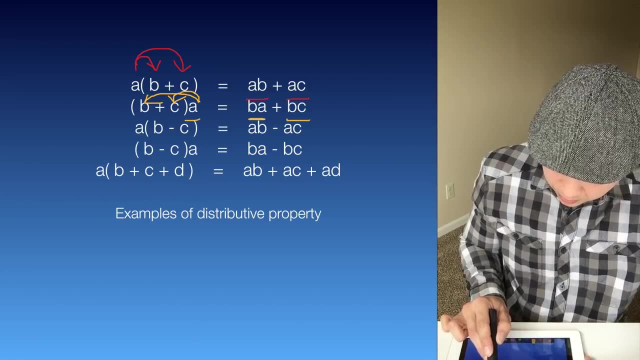 and then we have multiplication of b times a, and then we can distribute a to c And then we have: that should be a c. So this should be a b a plus c. So this should be a b, a plus c. 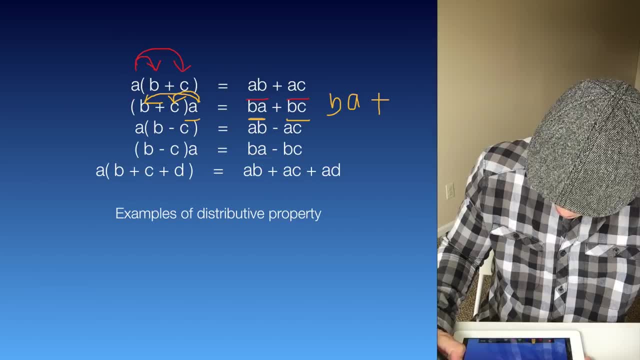 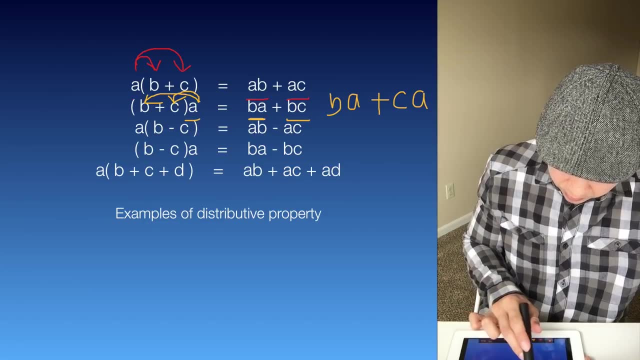 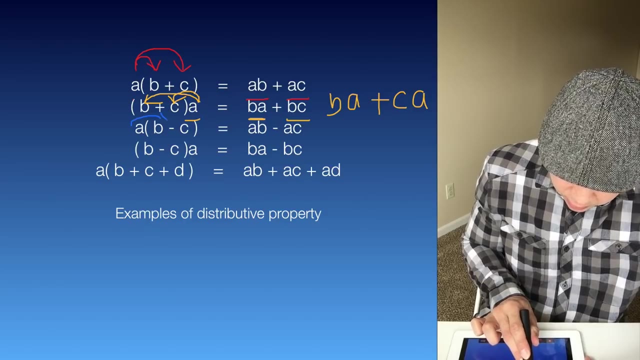 So this should be a, b, a plus c a. So now here we have b minus c times a, So we could distribute a to b, and then we distribute a to c, So we have a times b. 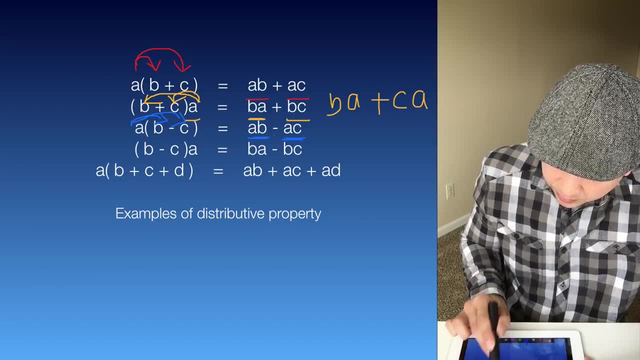 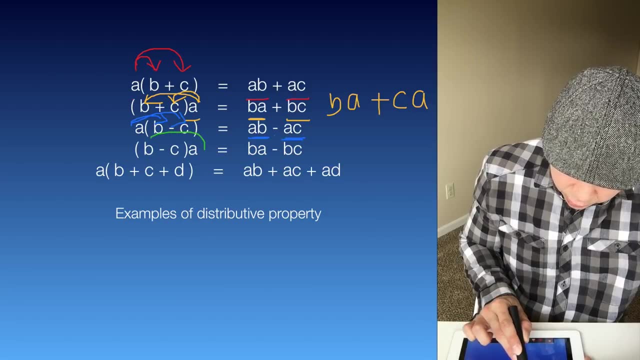 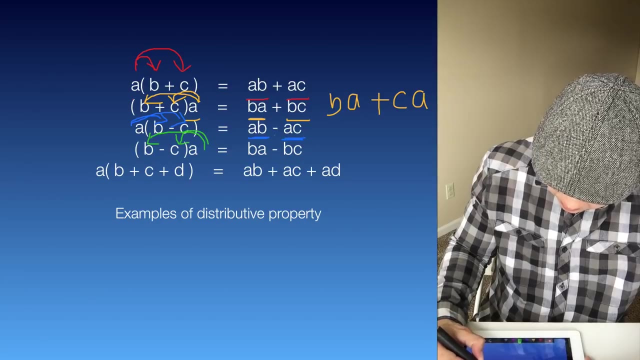 That gives us a times b minus a times c. So here we have b minus c times a. Now we could distribute a to b and then distribute a to c, So that gives us b a minus c a. 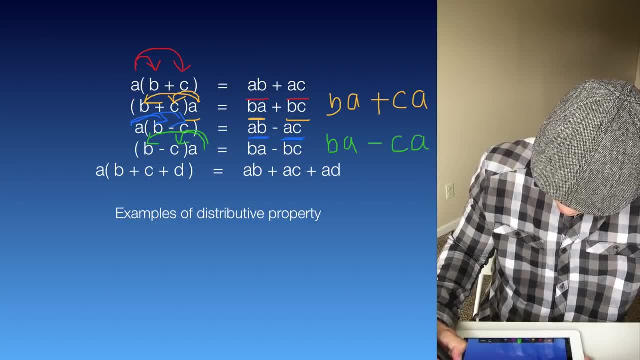 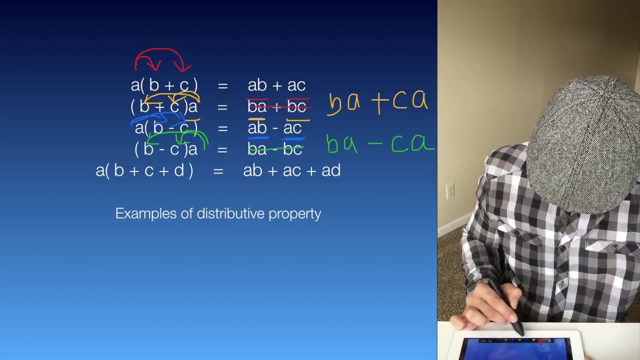 So that gives us b a minus c a. We just cross this out. So now here we have b plus c, a minus c a. So now here we have b plus c a. So now here we have b plus c a. 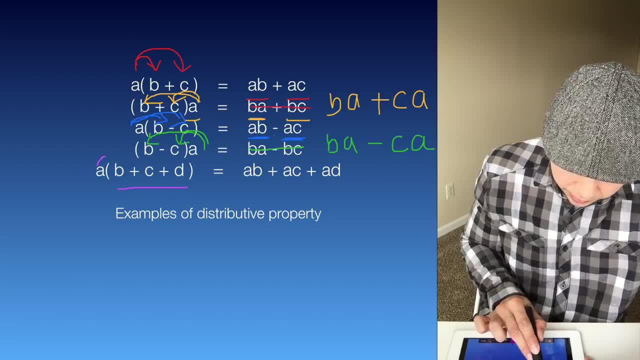 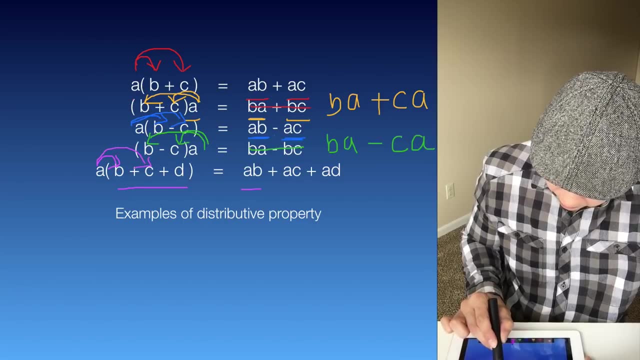 So now here we have b plus c, plus d times a. So when we distribute a to b, we have a times b. When we distribute a to c, we have plus a, c, And then when we distribute a, 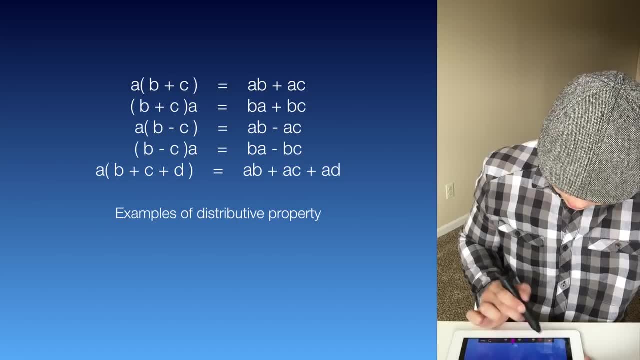 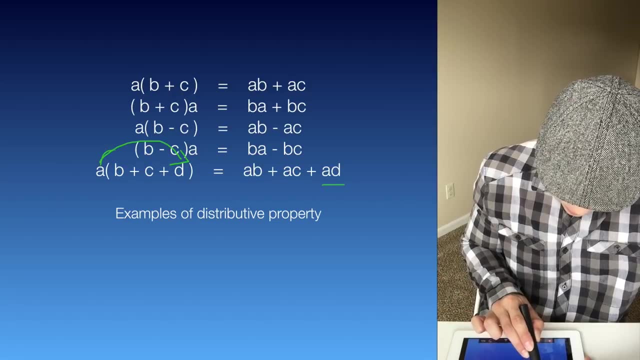 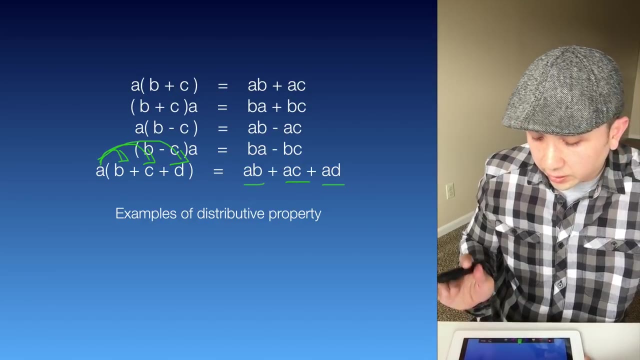 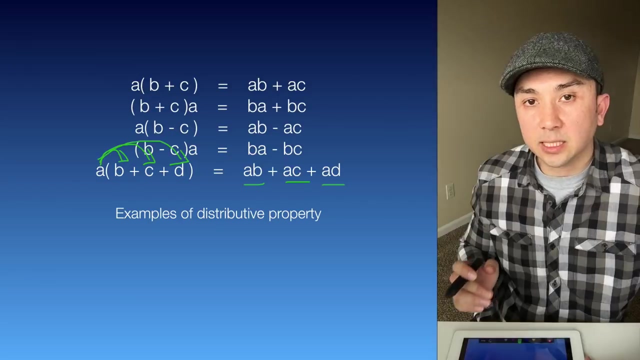 sorry about that. So when we distribute a to d, we have a- d, So a to b, a to c. So that's how we distribute a to b plus c, plus d, using the distributive property. So let's do an example. 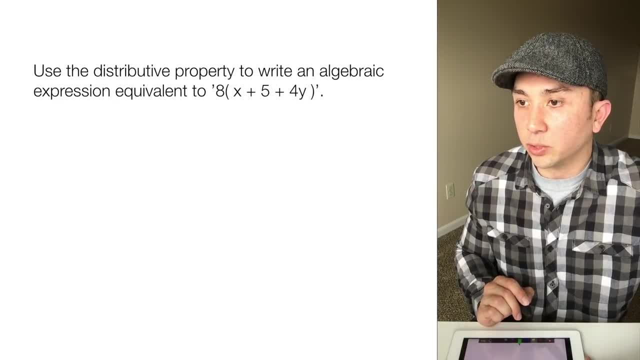 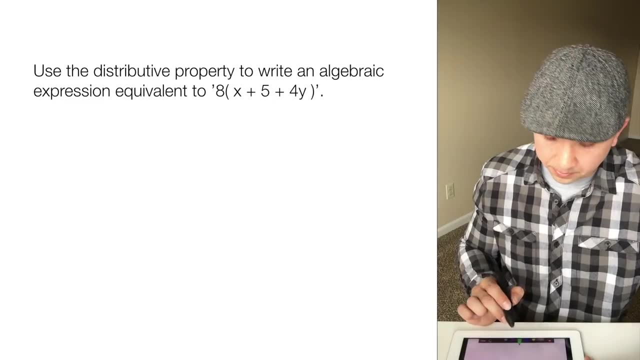 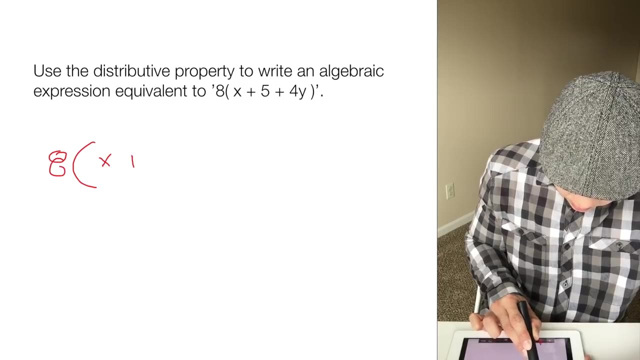 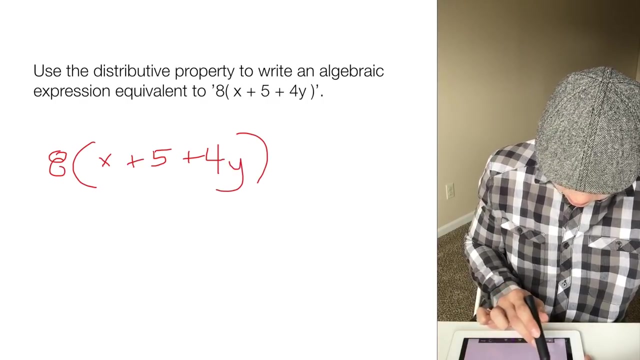 Let's use the distributive property to write an algebraic expression equivalent to eight times x plus five plus four y. So here we have eight times x plus five plus four y. So when we distribute eight to x, we have eight x. 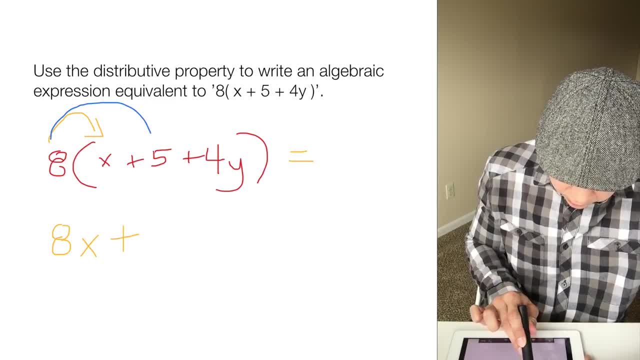 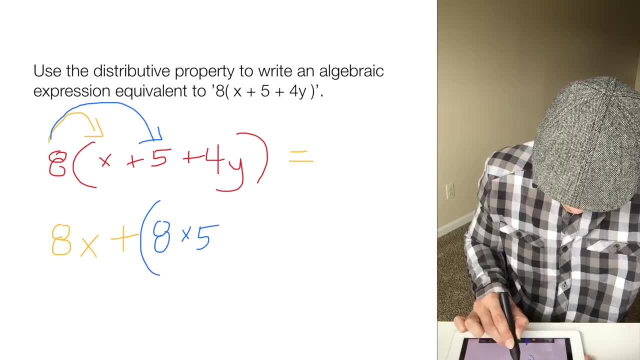 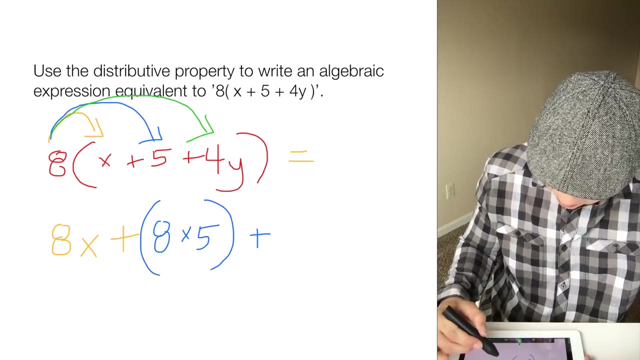 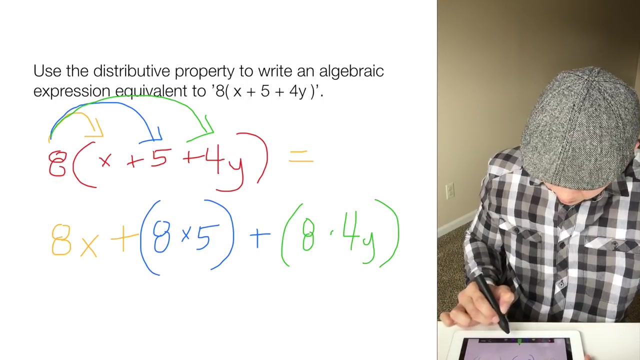 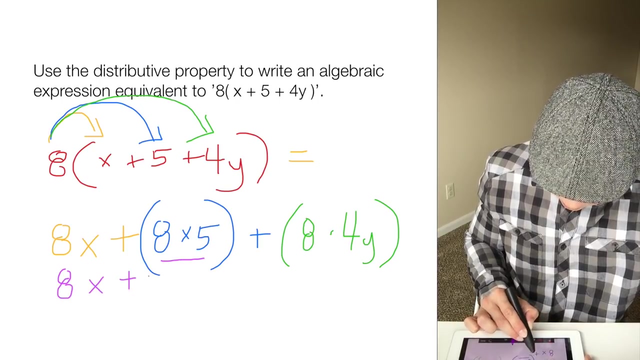 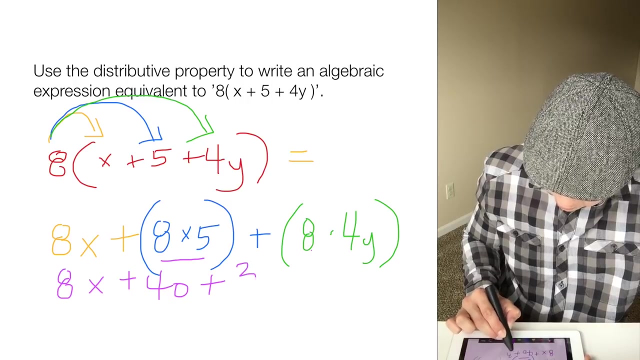 plus. distribute eight to five, we have eight times x 5 plus. and then we distribute 8 to 4y, we have 8 times 4y. Now we can simplify this as 8x plus 8 times 5 is 40, plus 8 times 4y is 32y. 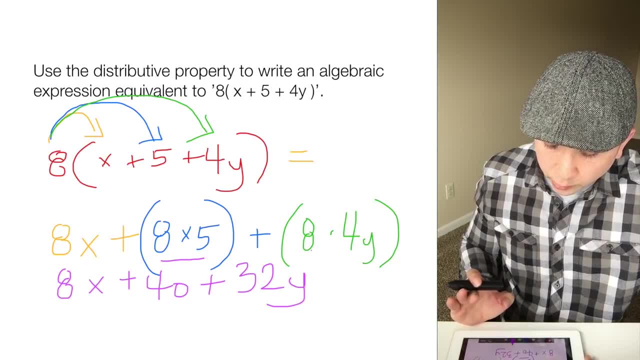 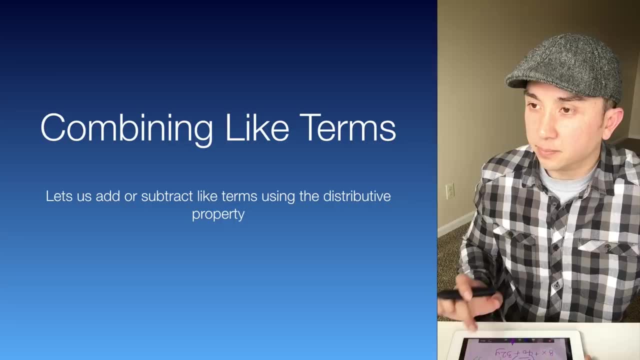 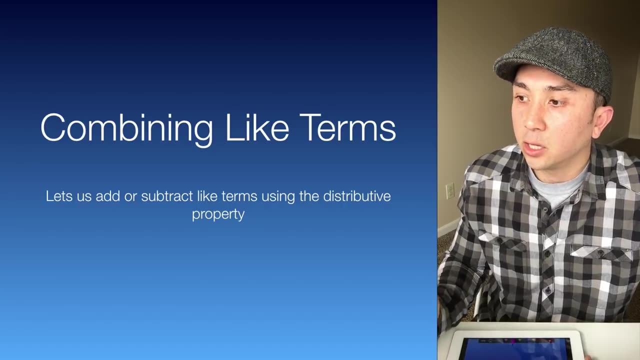 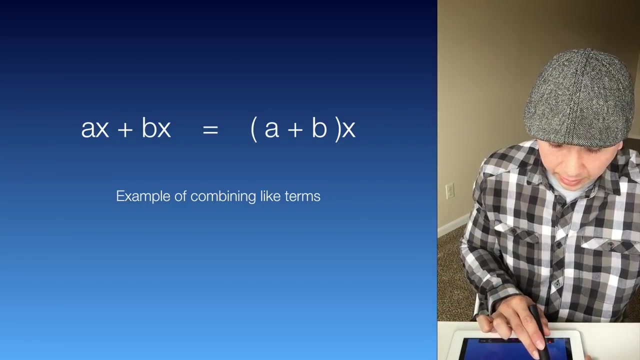 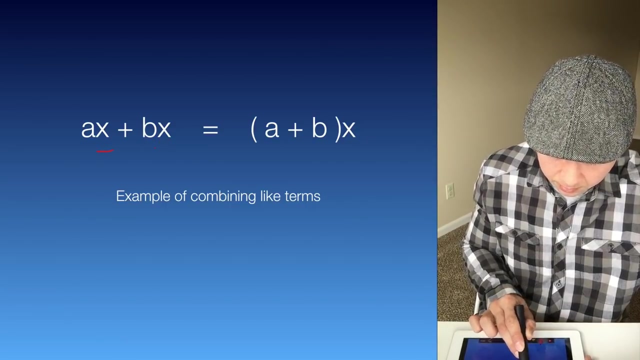 So that's how we distribute 8 to x plus 5 plus 4y using the distributed property. Now, combining like terms lets us add or subtract like terms using the distributed property. So here we have ax plus bx and our like terms are x raised. 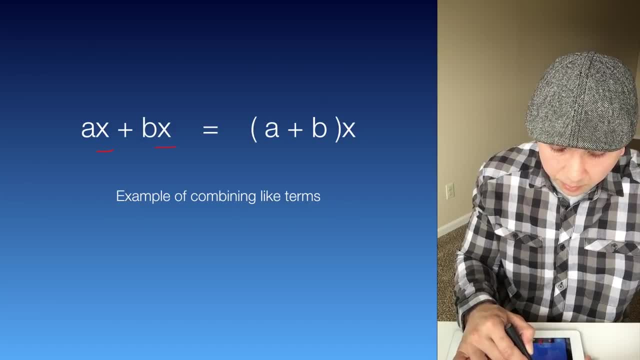 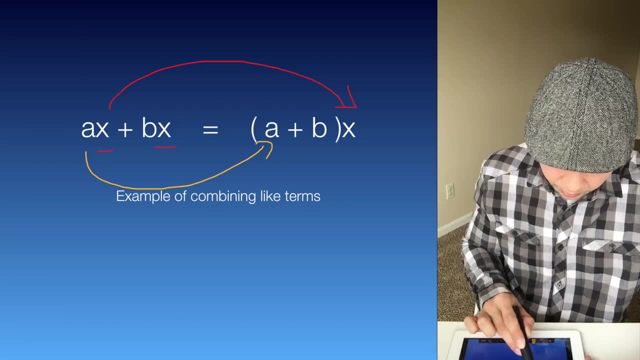 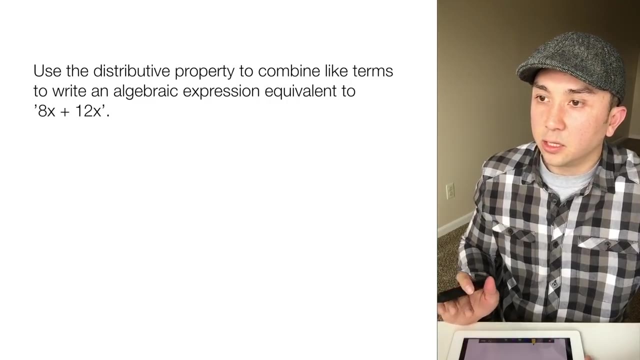 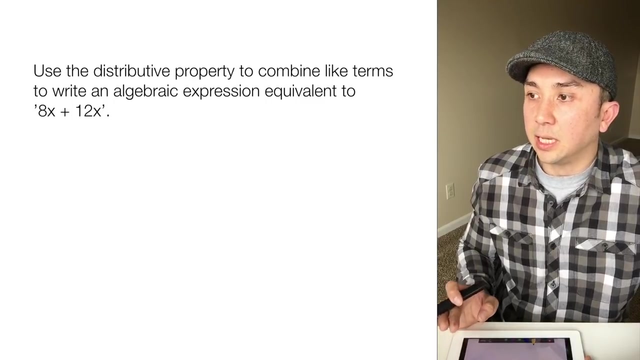 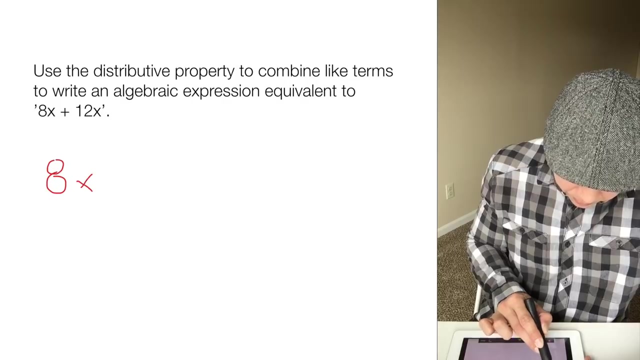 to the first power, So we can combine them into x and then just write. Let's do an example: Use the distributed property to combine like terms to write an algebraic expression equivalent to 8x plus 12x. So here we have 8x plus 12x. 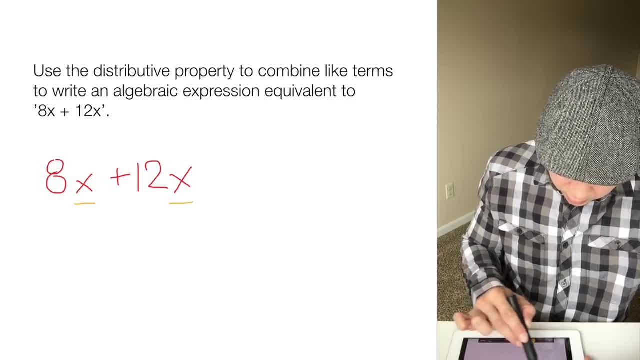 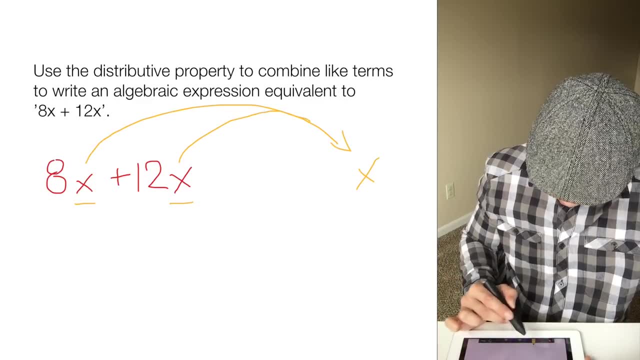 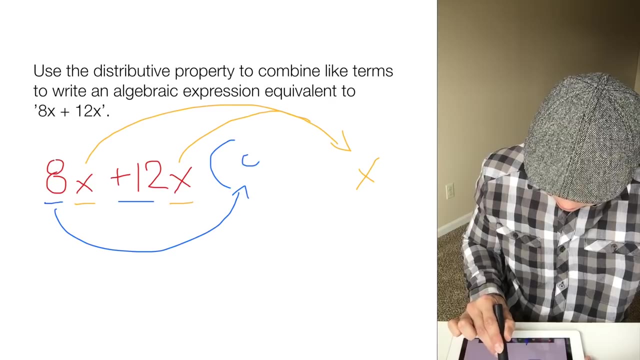 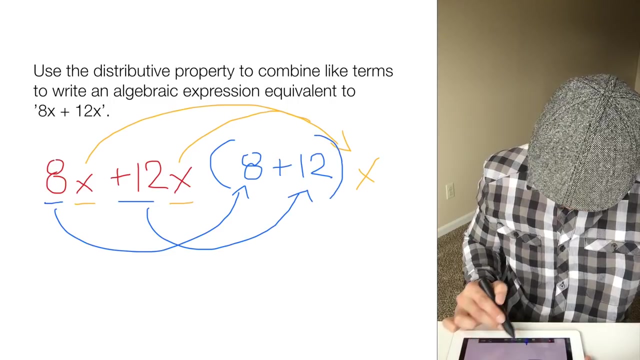 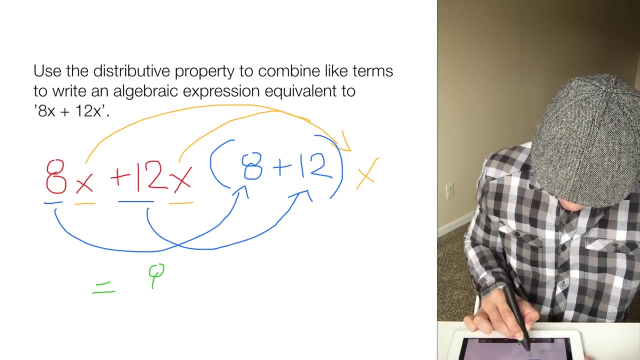 So our like terms are x, So that means we can combine them into just x. Now we can get our 8 plus 12 and write that here, So we just have 8 plus 12.. So we can write that down here for simplicity. 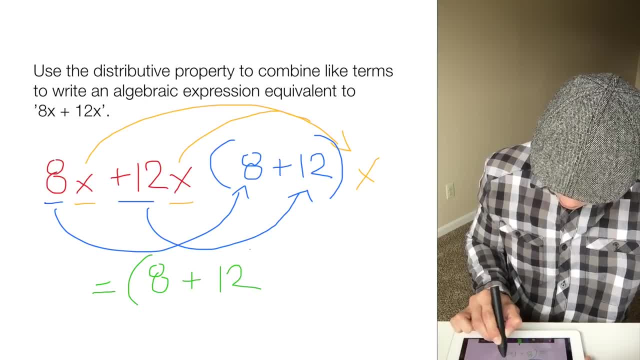 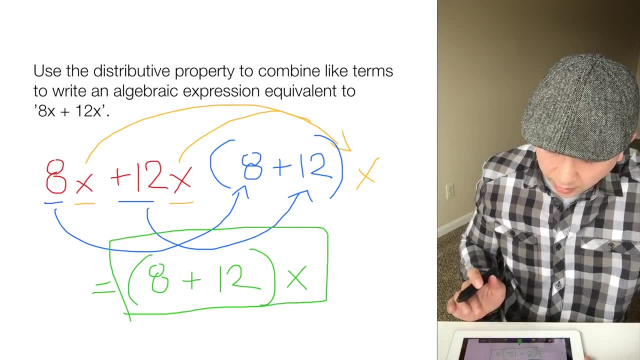 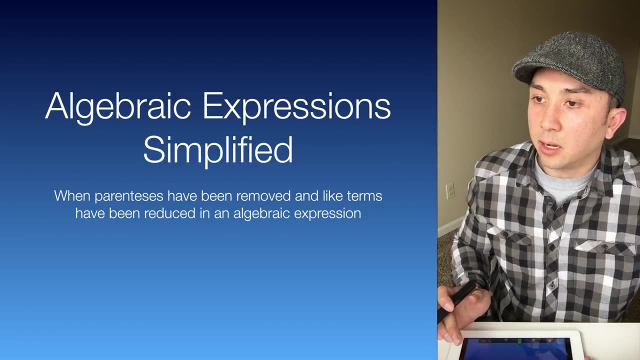 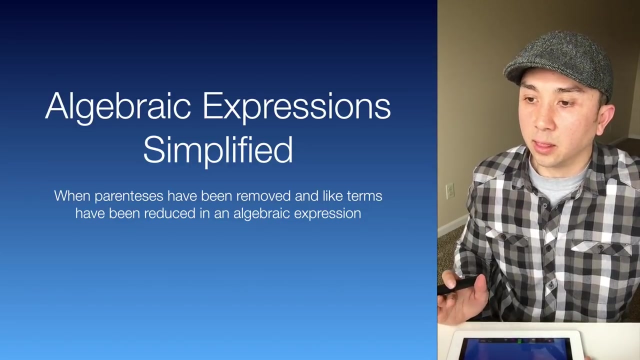 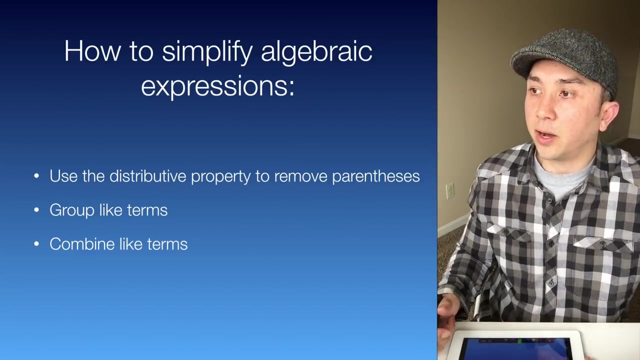 8. 8 plus 12 times x. So that's how we combine like terms using the distributed property. Now an algebraic expression is simplified when the parentheses have been removed and the like terms have been reduced in an algebraic expression. So here's how we simplify an algebraic expression. 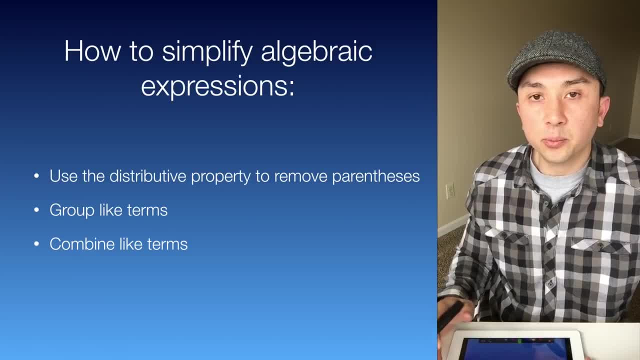 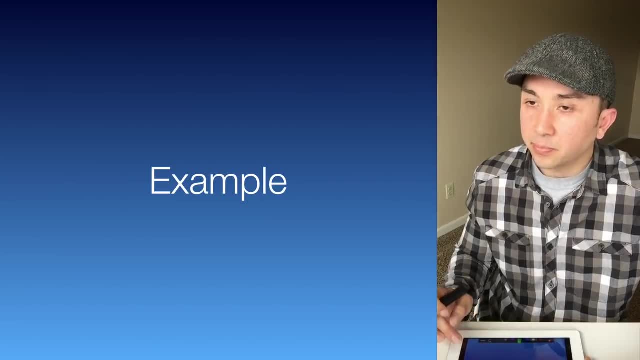 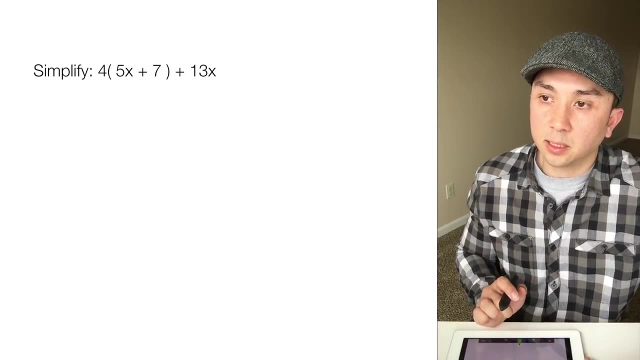 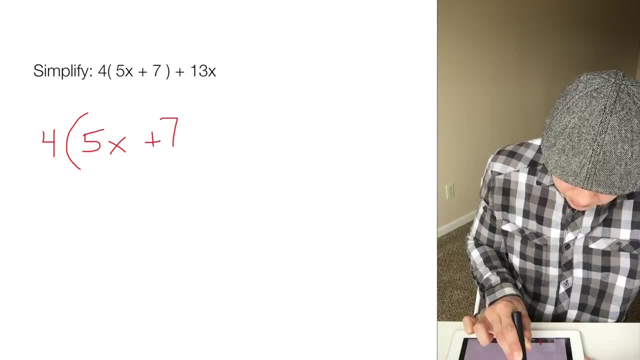 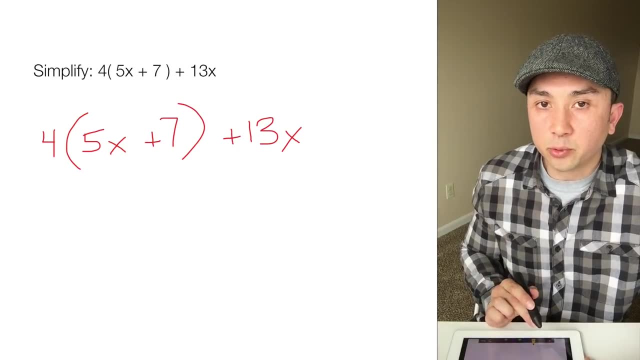 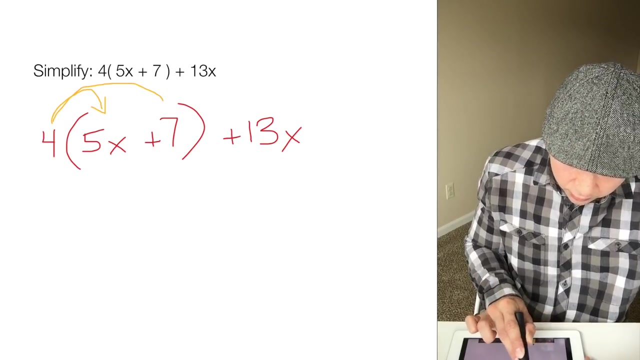 So here we have 4 times 13x. So here we have 4 times 13x plus 7 plus 13x. So the first thing we're going to do is use the distributed property to combine like terms. So we're going to distribute 4 to 5x and distribute 4 to 7.. 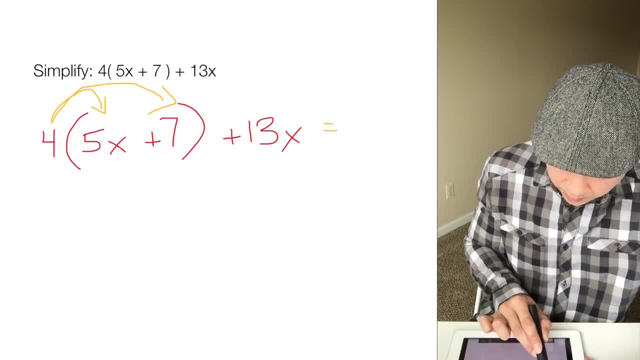 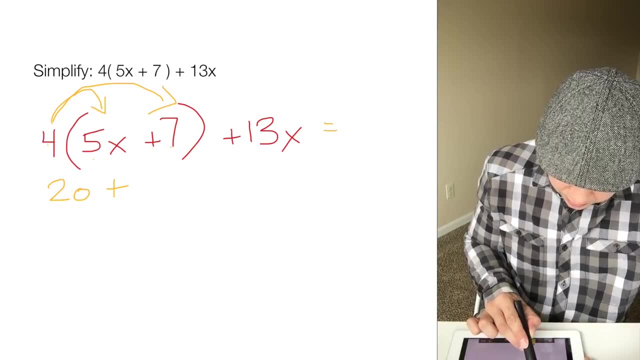 So that gives us: 4 times 5x is 20x plus 4 times 7 is 20x. So that gives us: 4 times 5x is 20x plus 4 times 7 is 28 plus 13x. 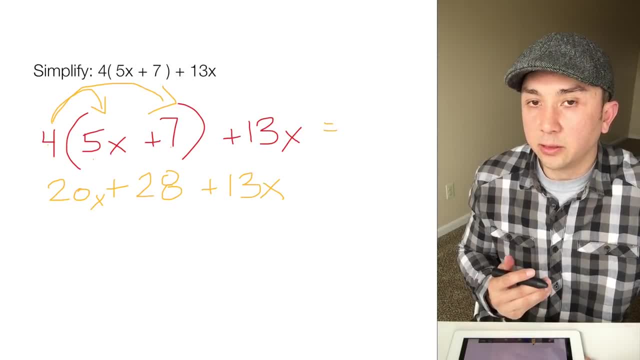 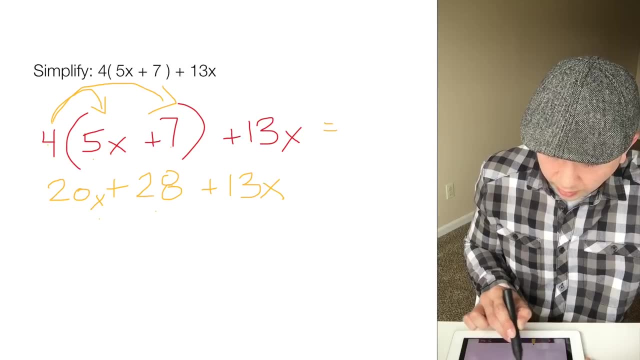 So we're going to combine like terms using the associative property. So know we can add 20x plus 28 plus 13.. So we know we can add 20x plus 28 plus 13 plus 4 times 5x is 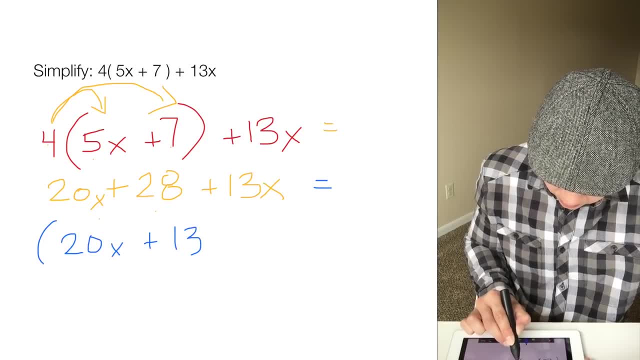 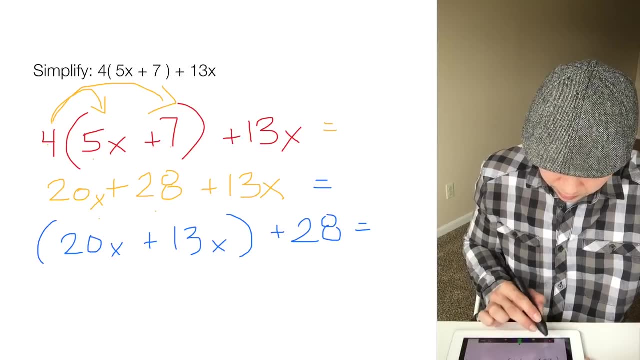 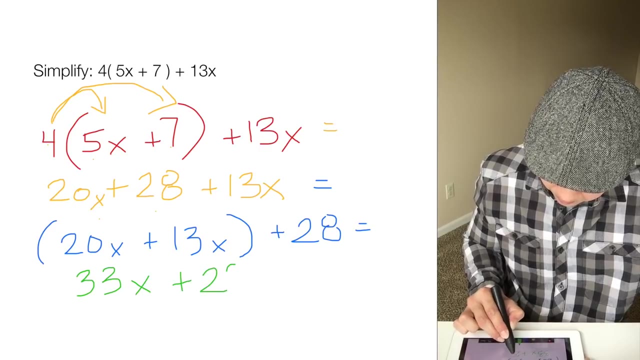 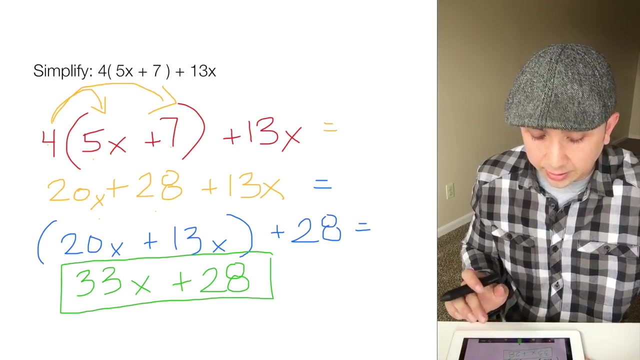 Or we can add 20x plus 14.. So we know we can add 20x plus 14.. 13x plus 28.. So here, 20 plus 13 is 33x plus 28.. So that's our answer. 33x plus 28 is a simplified